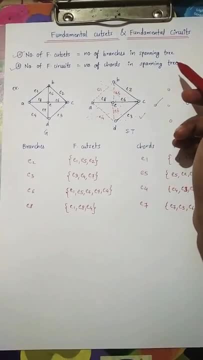 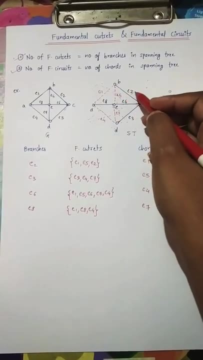 And we could get two or more cords for the cut set. So two cords would be E1 and E5.. Therefore, this would be our cut set, So it would be E1, E5 and E2.. Now for E3.. Where is E3?? 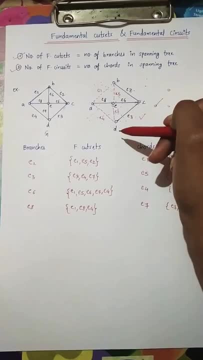 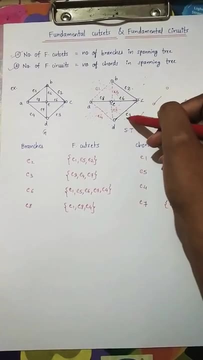 E3.. So for E3 branch, our cut set would be this one branch and these two other cords. So this can be our cut set. So for E3, E3, E4 and E7.. E3, E4, E7.. 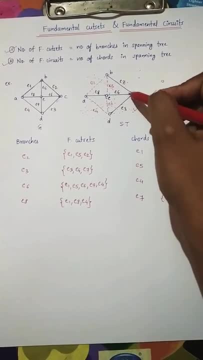 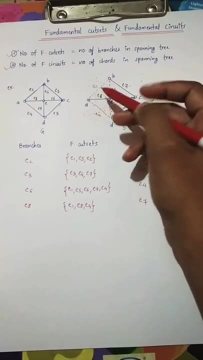 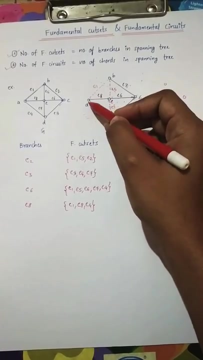 Now for E6.. E6 our cut set would be. E6 is our branch, which is present in the spanning tree And cords we could take. this could be our fundamental cut set. The cords are E1, E5, E7 and E4.. 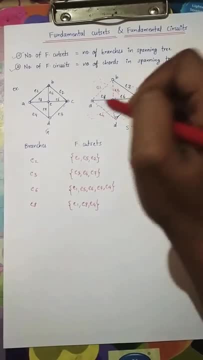 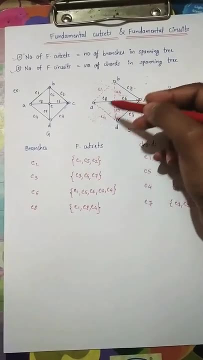 The cords can be more than two, but the branch should be one, necessarily only one. So E6 is our branch and there are four cords. So the cut set would be E1, E5, E6, E7 and E4.. 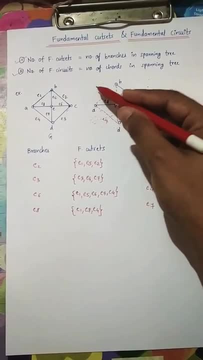 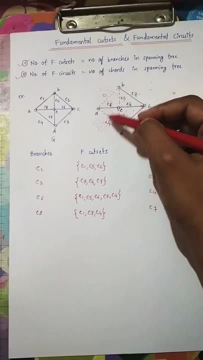 Now for E8.. For E8, we can have this cut set simply: E8 is our branch and these two would be our cords. So E1, E8 and E4.. E1, E8, E4.. Now coming to the cords and fundamental circuits. 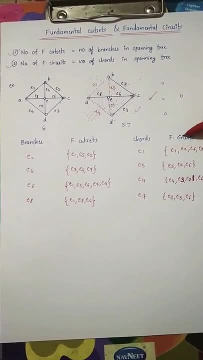 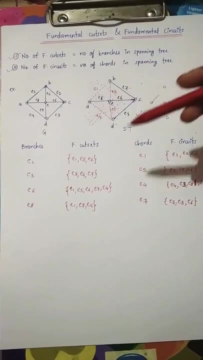 Cords. I have already explained you right now. So fundamental circuits. In the fundamental circuit the basic principle is that there should be only one cord. There can be more than one branches. The fundamental circuit concept is totally opposite of the cut set concept. 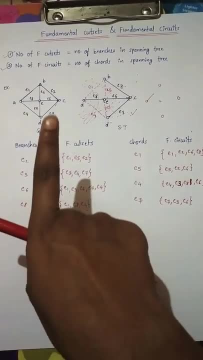 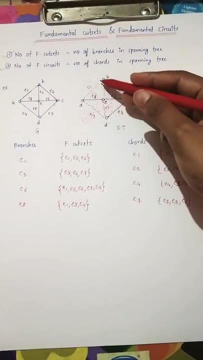 In cut set we are having, we need only one branch and in fundamental circuits we need only one cord. So the cords are which are not present in the spanning tree. the cords are E1, E5, E7, E4.. 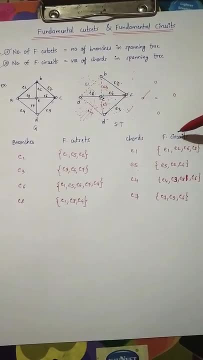 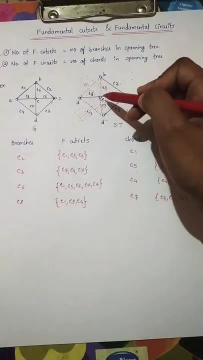 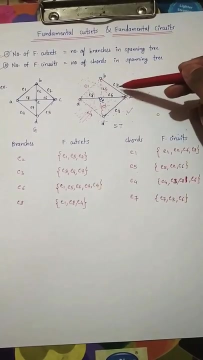 I have written it in here. So for cord E1, fundamental circuit would be: When we take E1, what circuit is forming? One cord and more than one branch. So these are our branches and this is one cord. So the circuit would be E1, E2, E6 and E8.. 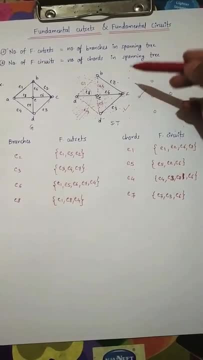 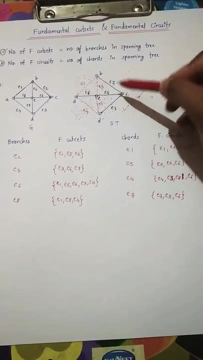 E1, E2, E6, E8.. This is our circuit For E5.. Where is E5?? This is E5.. Only one cord. There are two branches. More than one branch should be there, So we will take these two branches. 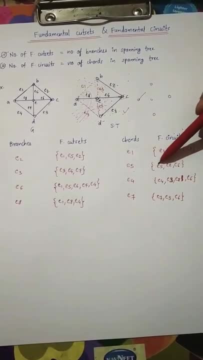 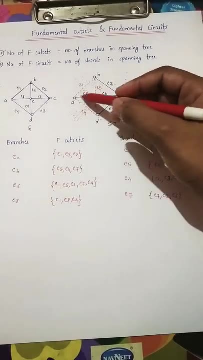 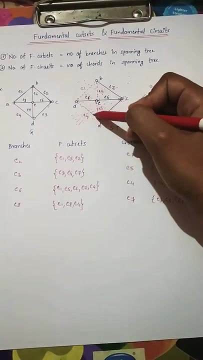 So E2, E5, E6.. E2, E5, E6.. This is our fundamental circuit for E5 cord. Now for E4.. E4, one cord more than one branches. Take these branches, See if you will consider this: E4, E7 and E8.. 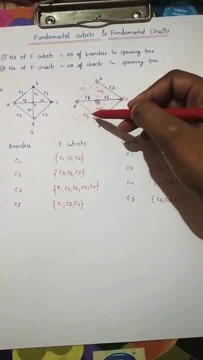 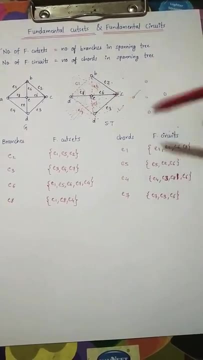 There are two cords, which is not possible. We need only one cord. So our circuit would be E4, E8, E6, E3.. E4, E8, E6, E3.. This is our fundamental circuit for E4.. 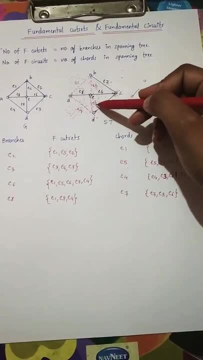 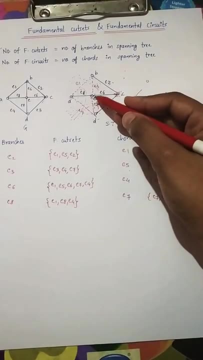 Now for E7.. Where is E7?? This is our E7.. Sorry, it's not visible, neatly So for E7.. We need only one cord and two branches. So E7,, E6, E3.. E7,, E3, E6..